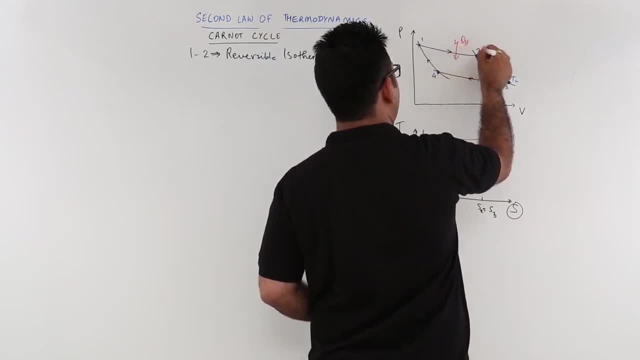 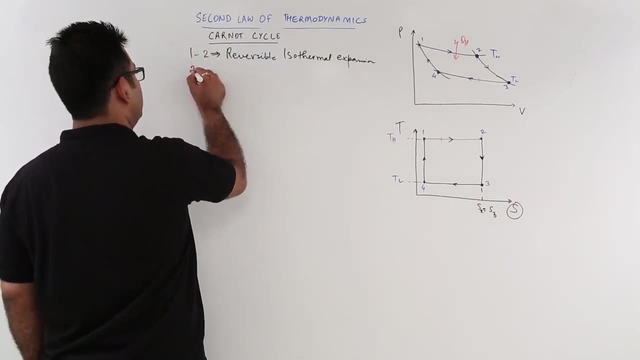 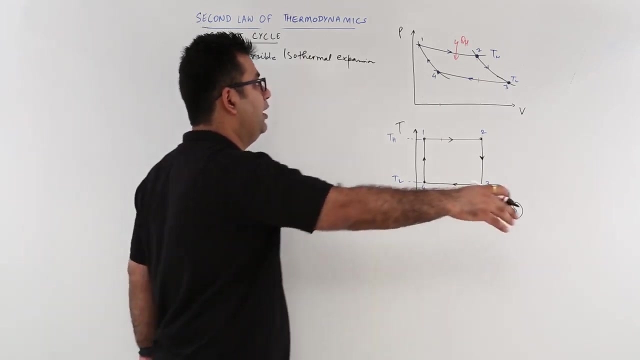 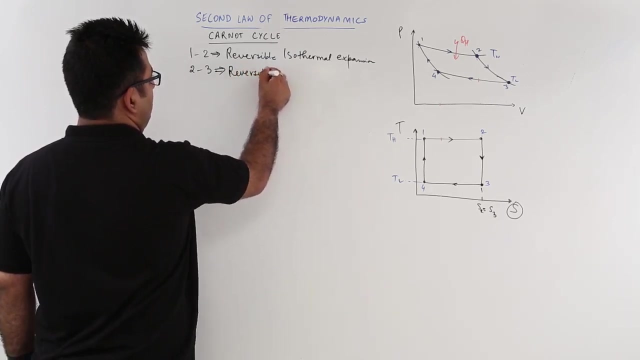 So you have some heat absorption at temperature TH. Then we come to Process 2, 3. Now all the processes in this cycle are reversible. This means they can be retraced exactly to their initial state. So this is reversible. This is reversible. 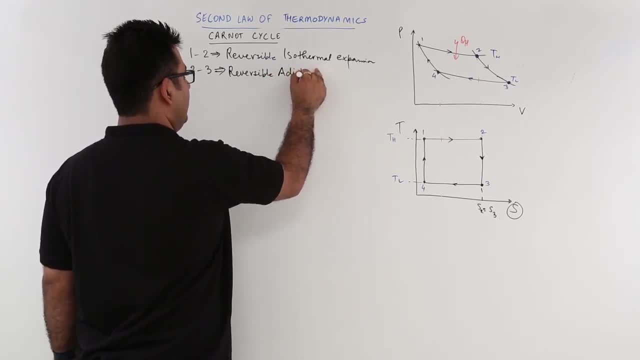 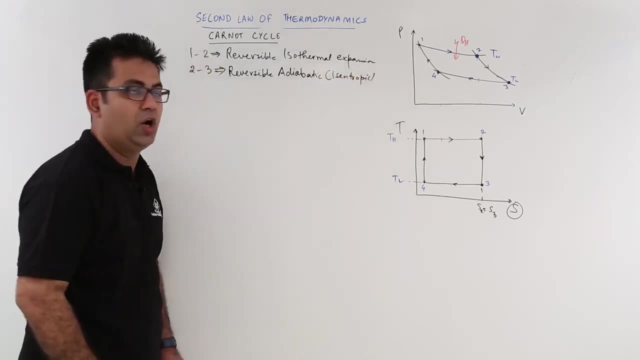 Adiabatic Now, reversible adiabatic means it is an isentropic process. Same entropy: Reversible adiabatic or isentropic. Again it is an isentropic process. Again it is expansion. You can see that. 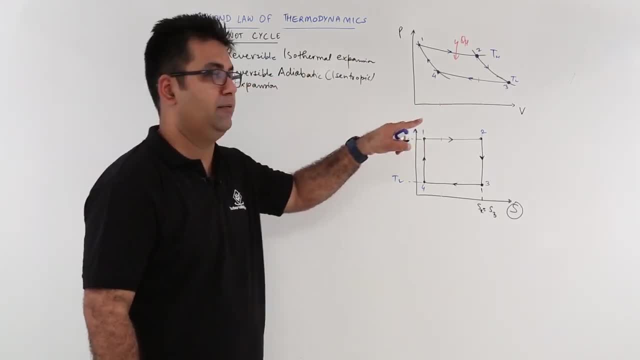 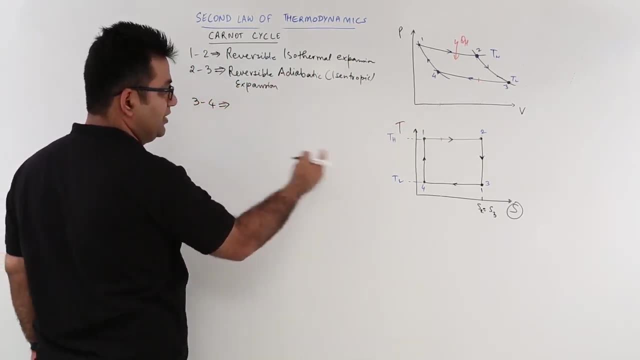 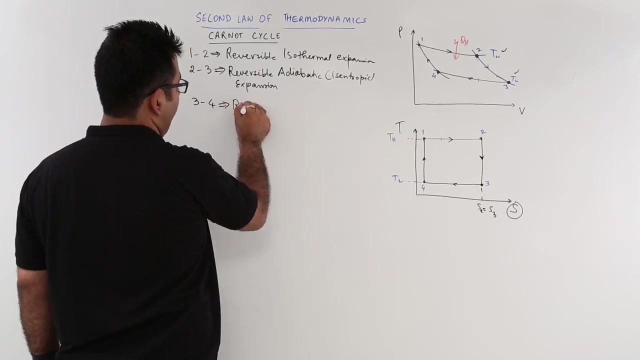 Now, in this there is no heat interaction because it is an adiabatic process. Now we come to 3 to 4.. 3 to 4 again becomes isothermal. There are two temperature limits, TH and TL, So this becomes reversible. 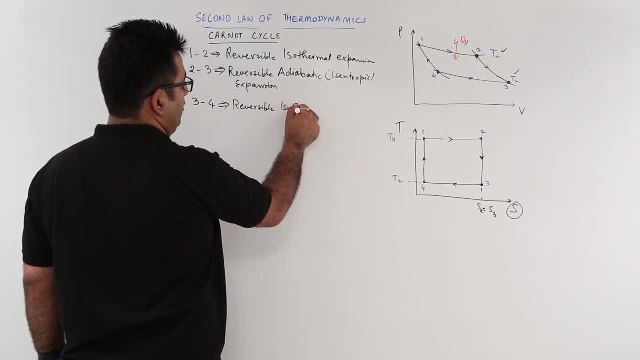 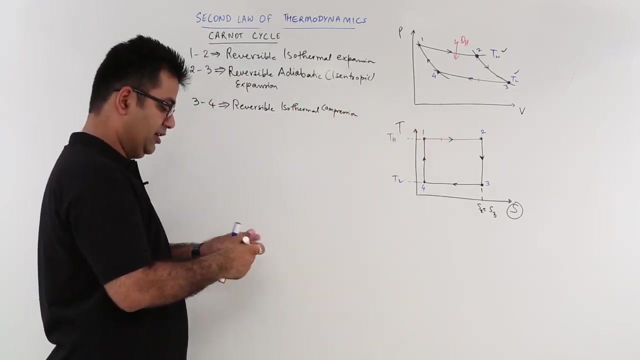 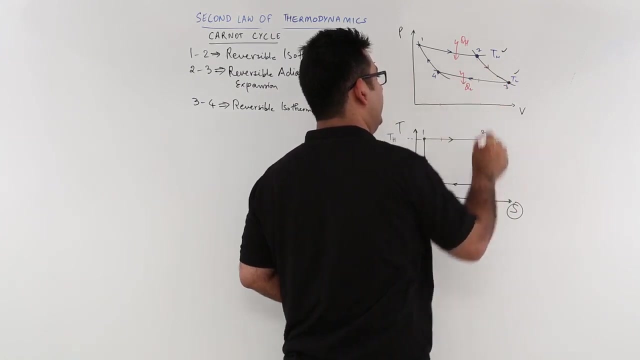 Reversible Isothermal Compression. Reversible isothermal compression: So because it is being compressed, so the gas inside becomes hot, So it will now reject heat. So this is the heat rejection at temperature TL. Okay, You will have some heat. 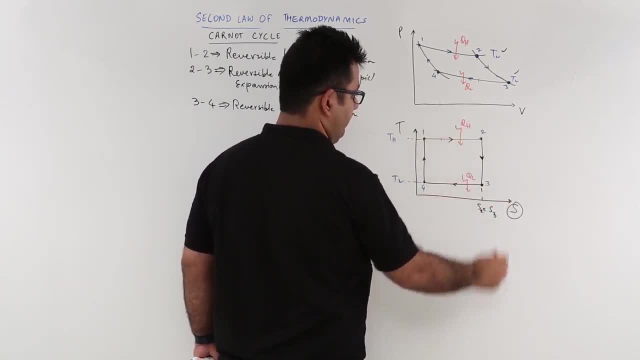 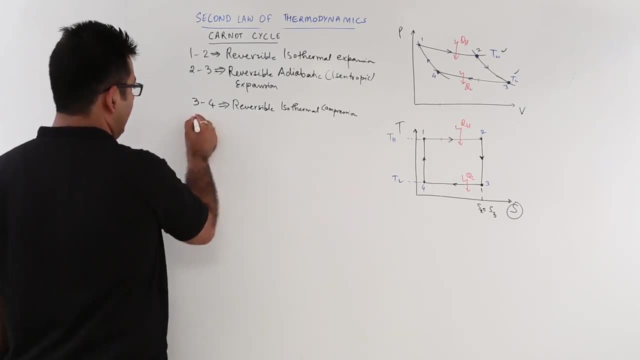 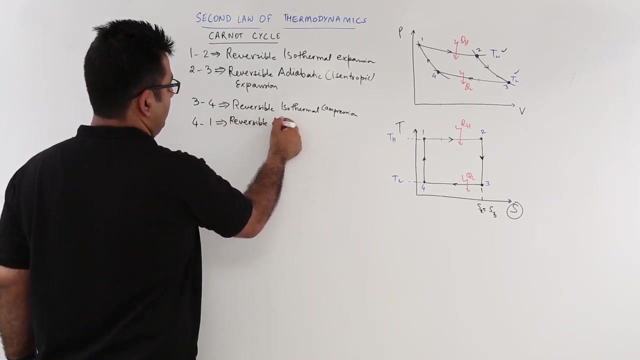 Over here, Over here, And some heat over here. Okay, Let us move ahead Now. 3 to 4 is isothermal compression, And then 4 to 1 it again becomes reversible adiabatic, Reversible adiabatic. 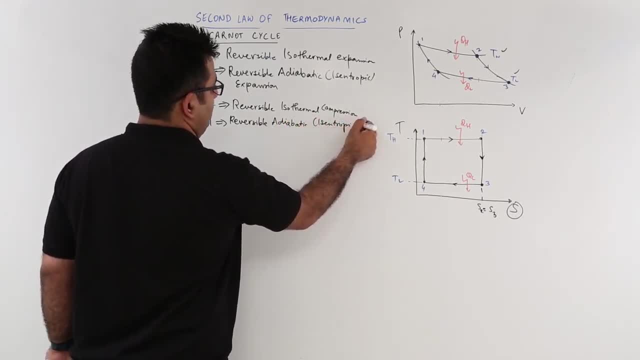 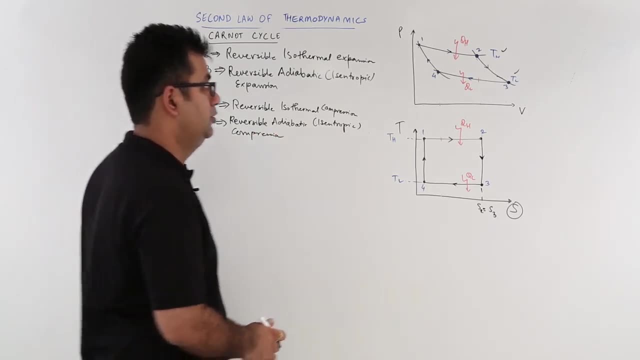 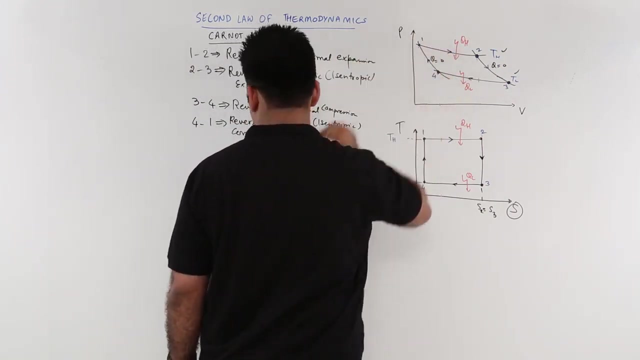 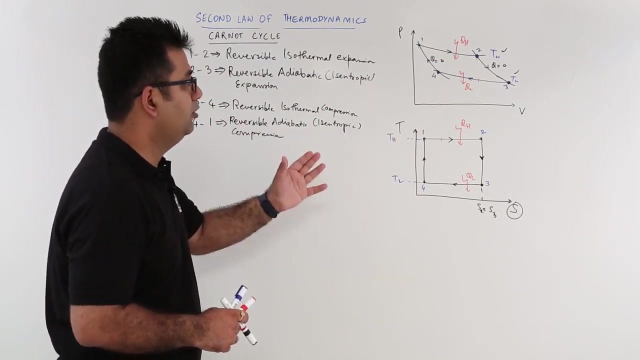 Or we also call it isentropic compression. Okay, Now let us look at the mathematical value for it. So 2, 3 q 0, 4, 1 q 0.. Okay, Let us look at the values. So for 1, 2, it is an isothermal. you know process. 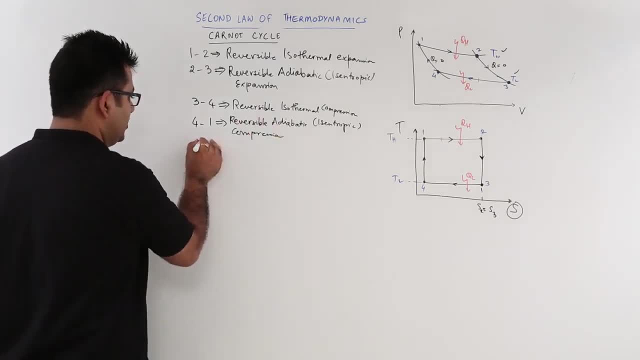 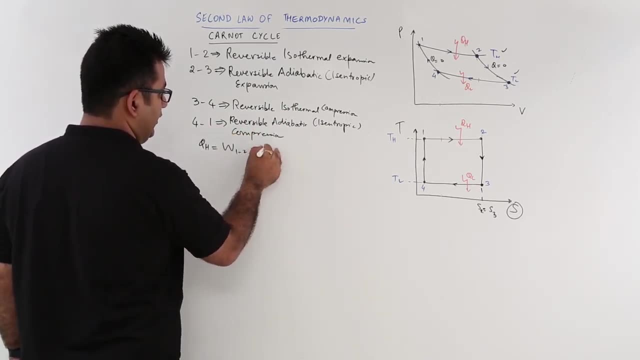 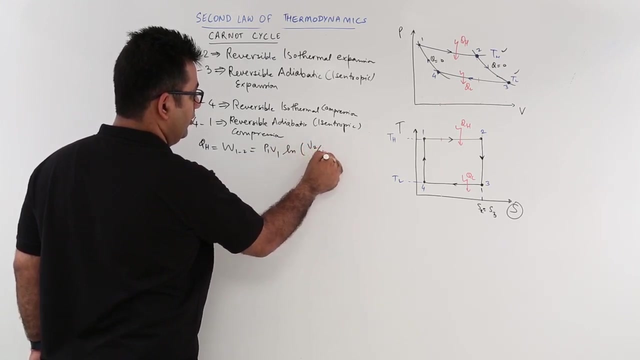 So q will be equal to w. So q h is equal to w 1- 2.. That is equal to That is equal to what? That is equal to p 1 v 1.. Into natural log of v 2 by v 1.. 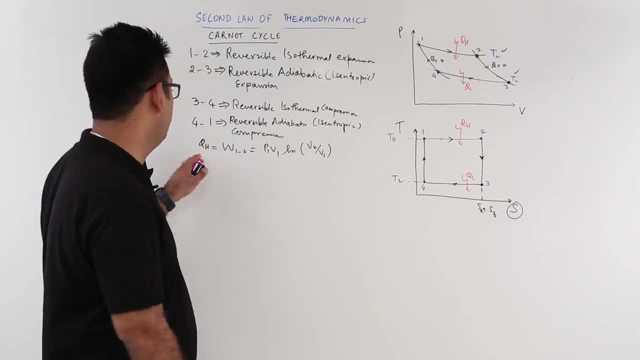 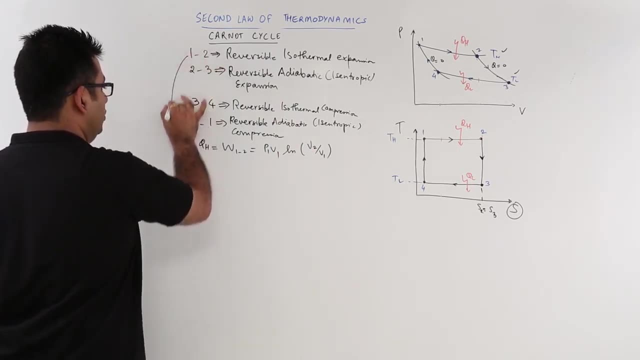 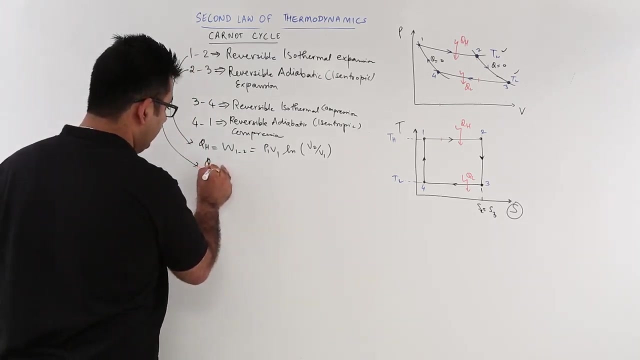 So this is the value of the isothermal work, which is equal to the heat absorption at temperature TH. Okay, Now this is for 1- 2.. Let us look at the same thing for 2, 3.. Now for 2, 3. that is q, 2, 3, it is u. 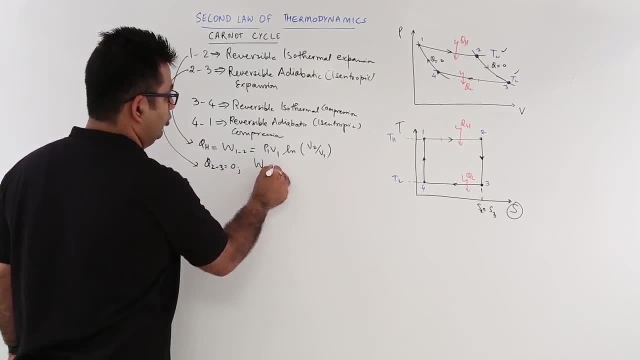 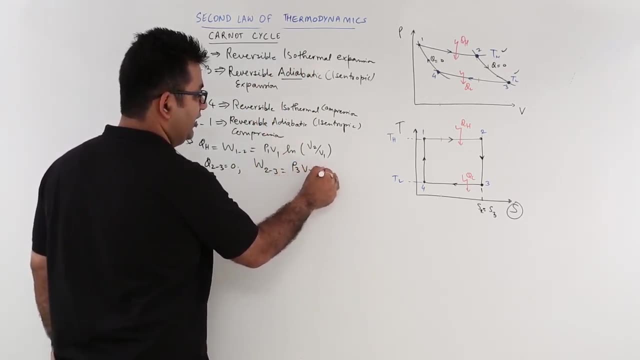 Let us find out the work value. So that is w 2, 3.. Now it is an adiabatic, Now it is an adiabatic process. For adiabatic, you have p 3 v 3 minus p 2 v 2 by gamma minus 1, assuming we have air as 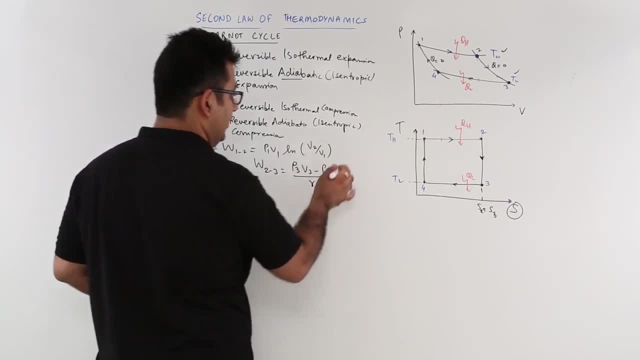 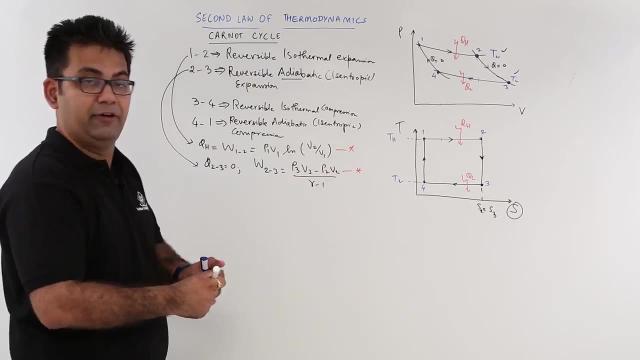 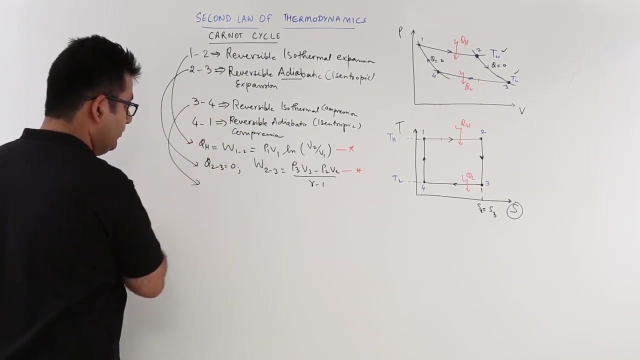 our working fluid. So you can now see that these are, you know, similar or you can say, quite familiar kind of expressions that we are using over here. Now let us come to process 3, 4.. For process 3, 4 q l will be equal to w 3, 4.. 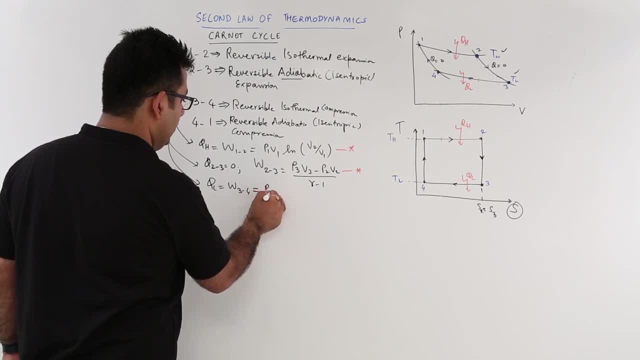 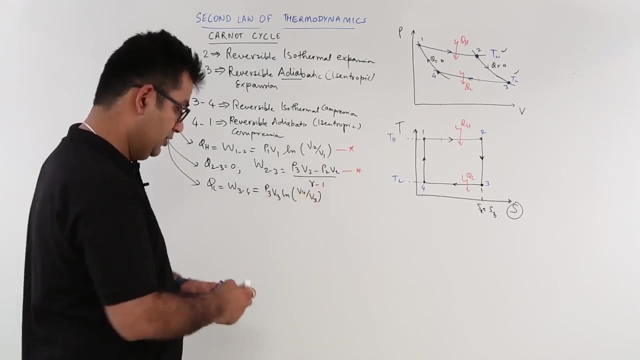 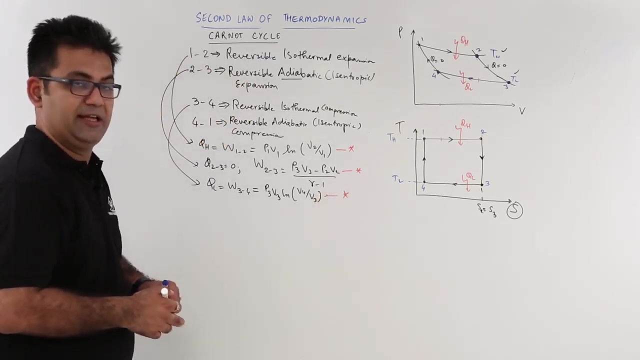 Isn't it? And that would be equal to p 3, v 3, natural log v 4 by v 3.. So that is again isothermal work, wherein the isothermal work and the heat lost are same. Now we come to 4: 1.. 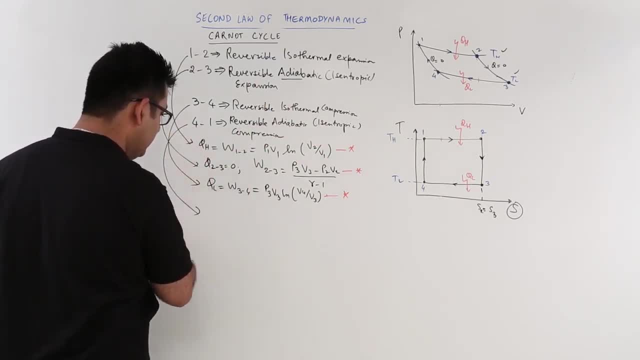 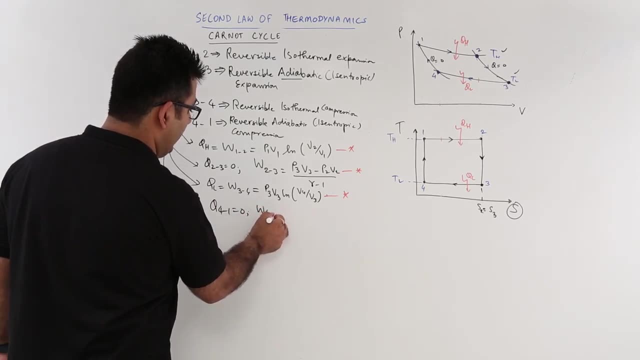 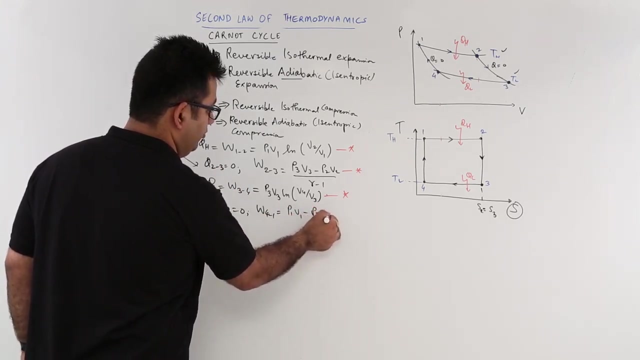 So for 4: 1 you have heat as 0. There is no heat interaction and w 4 1, which is again an adiabatic process. This becomes p 1 v 1 minus p 2 v 2. This is 4.. 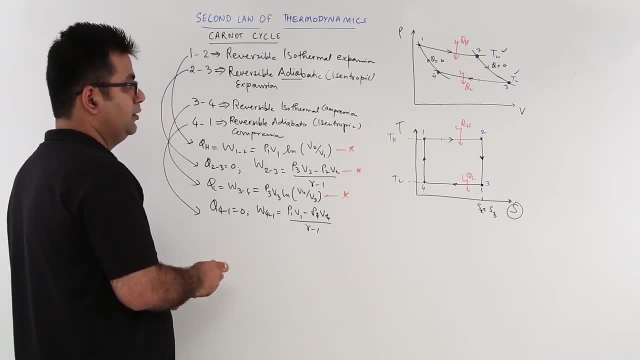 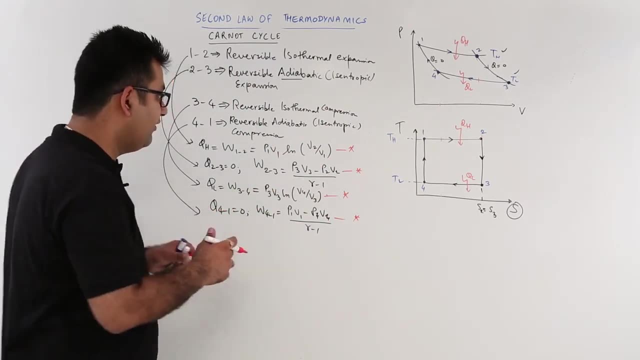 Okay, So these are the mathematical relations For the work and the heat values. Now let us derive an expression for the efficiency of the Carnot cycle. Hope you had learned anything. If you have, then do not forget to subscribe to eC 얼�ler, because will continue their. further lectures Open the.